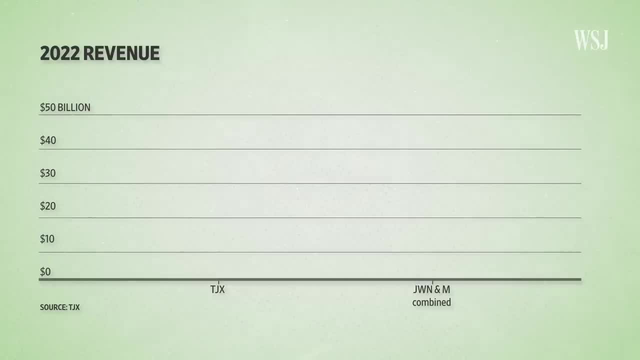 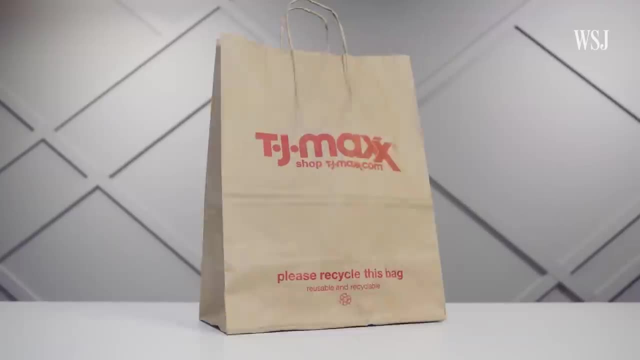 In 2022, TJX, which owns TJ, Maxx, Marshalls and HomeGoods, brought in almost $50 billion in sales revenue, more than Nordstrom's and Macy's combined. And the secret to its success? The company isn't shifting most of its business online or using big data to figure out what 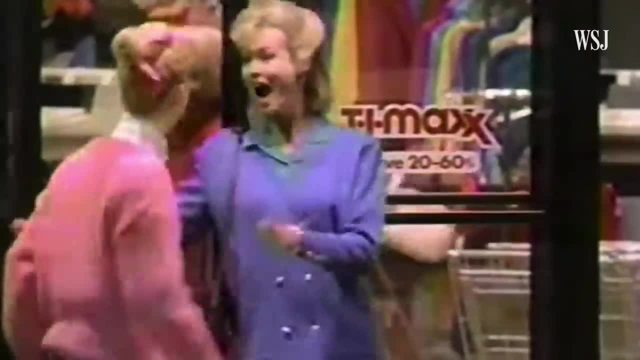 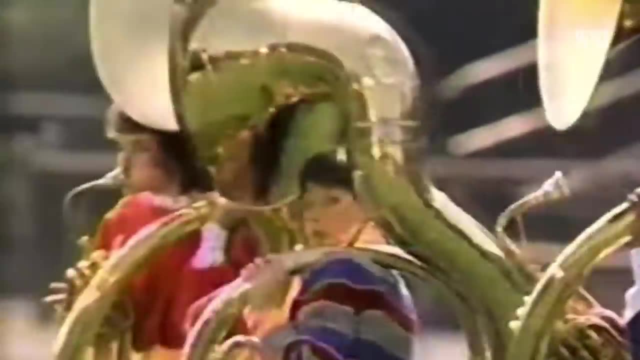 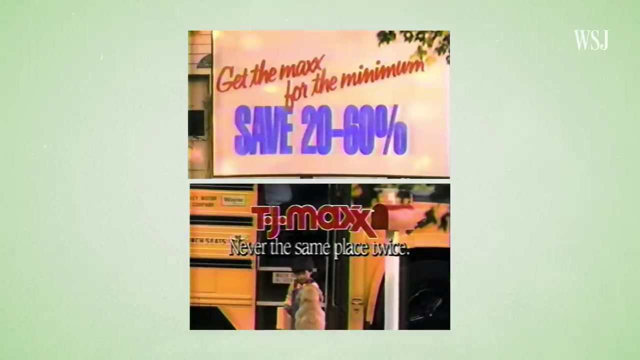 shoppers want. Instead, it's sticking to a decades-old playbook. This is the economics of TJ Maxx. There are really two components to TJ Maxx's strategy: the bargain and the hunt. One way TJ Maxx gets discounted goods is by buying excess. 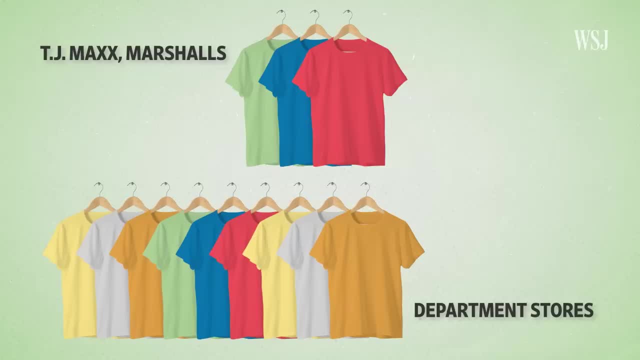 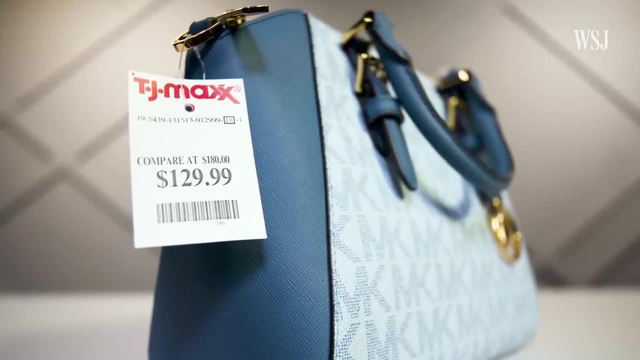 merchandise and cash. It's also a way to get canceled orders from other brands and retailers. Essentially, it takes advantage of surplus and waste in the retail system. This allows the company to sell its merchandise generally around 20 to 60% below regular retail prices. But there's a catch. 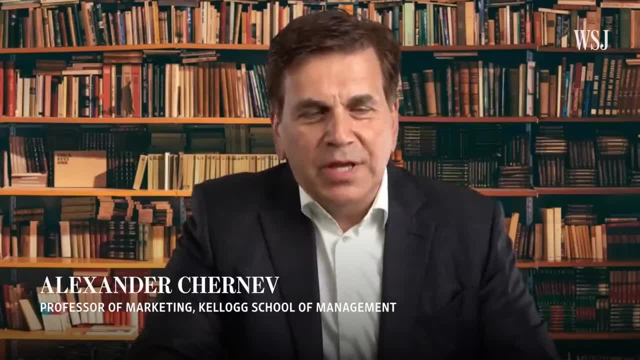 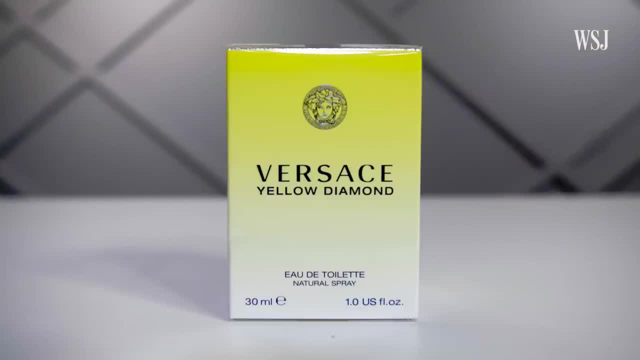 Just the fact that the price is low is not enough. What you need is also a reference price, because people don't know how much things cost. That's where Alex says something known as the anchoring effect comes in. At TJ Maxx, most items have two prices. 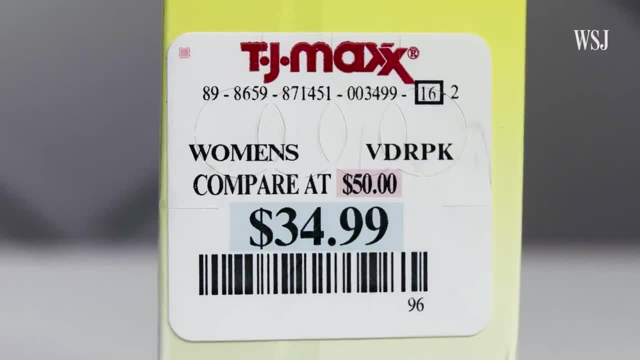 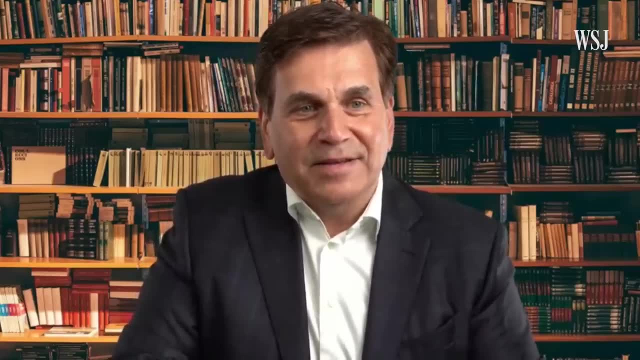 The TJ Maxx price and a comparison price. People anchor in the regular price and then they see exactly how much of a deal they're getting And this way they really understand what the value is that TJ Maxx provides to them. Take these rag and bone shorts. 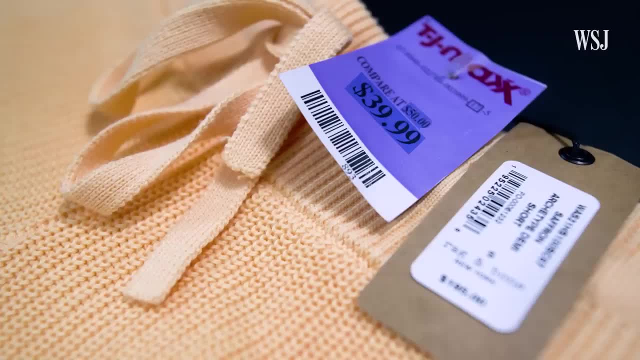 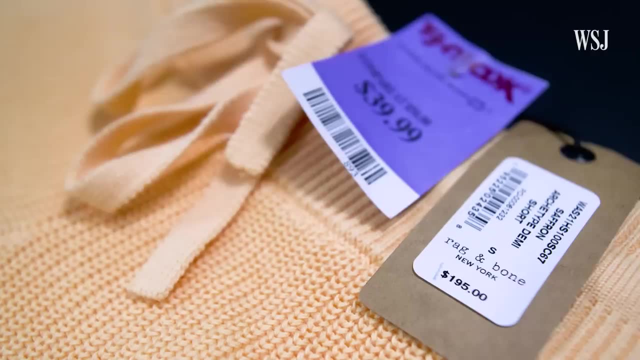 A TJ Maxx in Manhattan sold them for about $40, with a comparison price of $50. That's a 20 percent discount. But the original price tag happened to be on these shorts and it lists the price as $195.. That would be around an 80 percent discount. 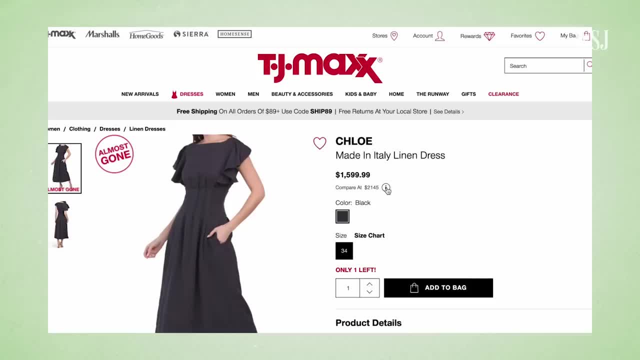 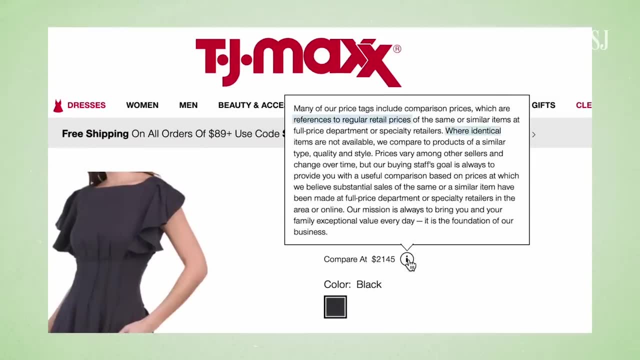 And that comparison price is really just an estimate. On TJ Maxx's website there's a message next to the comparison price that says these prices are references to regular retail prices Where identical items are not available. we compare to products of a similar type, quality and style. 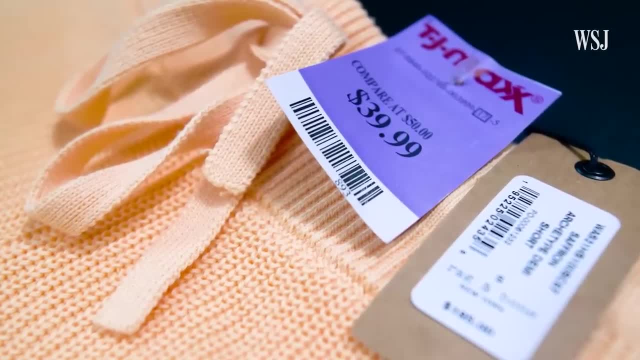 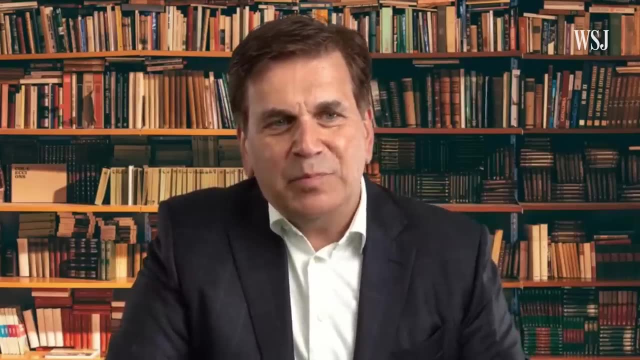 These price tags aren't the only way TJ Maxx helps customers feel like they're getting a bargain. The whole positioning of TJ Maxx is that if we give you brand names for less, And the reason why it's important is because very often when you see low price, 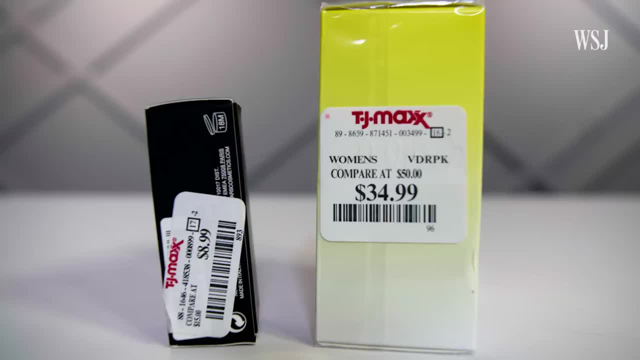 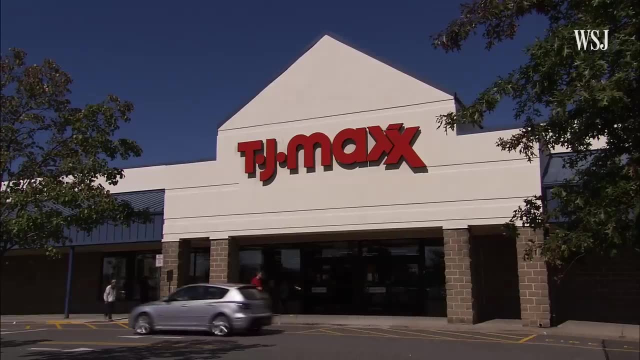 you think it's low price because the quality of the product is low. But if the customer knows and trusts the brand, then they won't assume the price is low because it's a bad product. Instead, Alex says they'll attribute it to TJ Maxx's ability to get discounted goods. 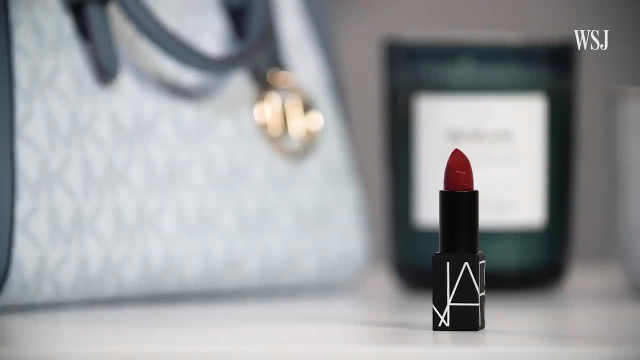 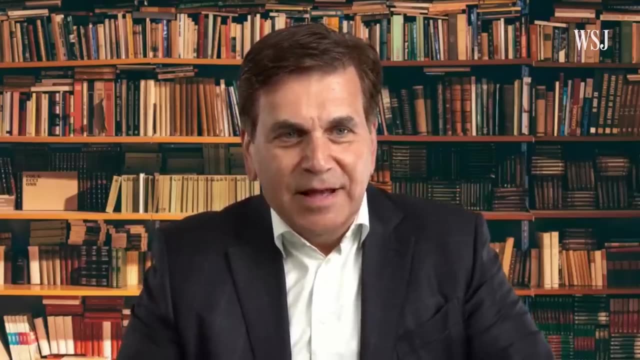 And because people often expect name brand items to be more expensive. the brand itself acts as an anchor. Emphasizing the fact that, as a customer, you're getting a deal makes people feel good. It's not only I'm getting a low price, but I'm actually getting a deal. 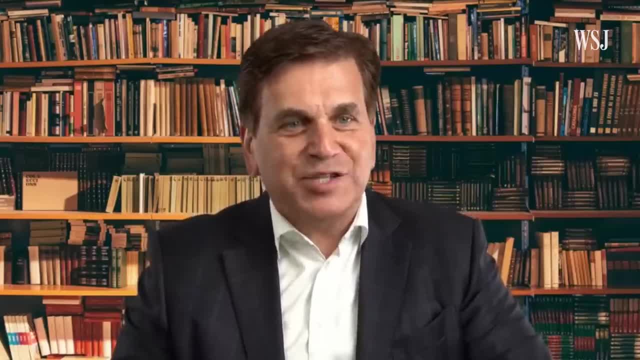 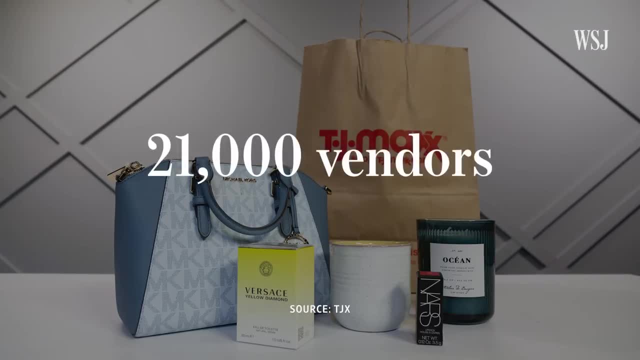 which makes people feel good about themselves, that they're smart shoppers. TJ Maxx says it gets its goods from about 21,000 vendors, and the inventory in its stores is constantly turning, So, as a result, people tend to go more often to this type of stores. 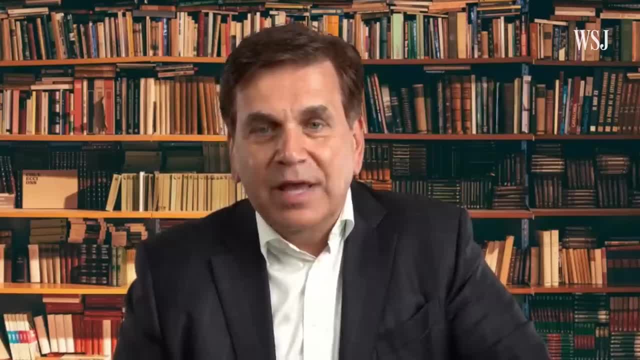 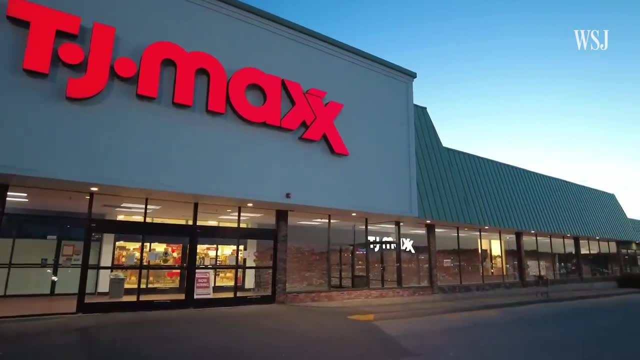 and also spend a little bit more time in the store in search of something. Across its companies, TJX employs more than 12,000 people. TJ Maxx has over 1,200 buyers that each control millions of dollars and has authority to cut deals on the spot. 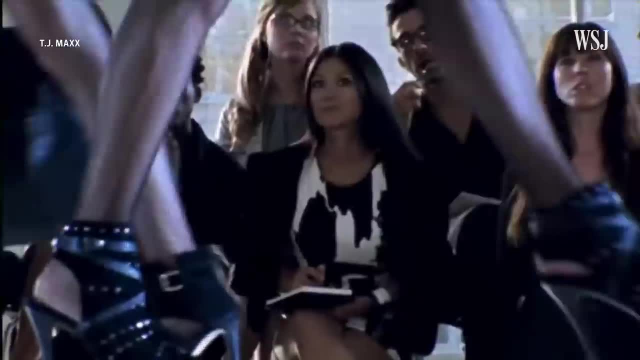 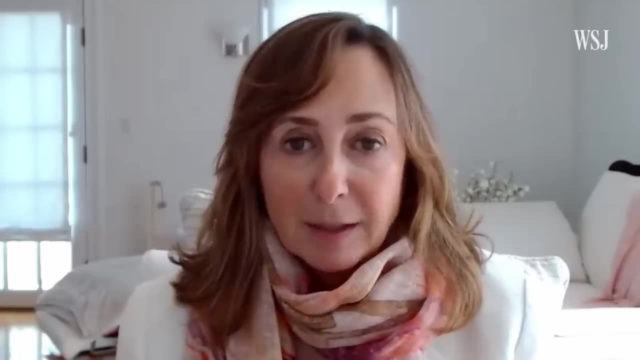 As a buyer for TJ Maxx, I'm always on the hunt. Let's say, you have a bathing suit brand and it's right before Memorial Day weekend and they're stuck with extra bathing suits. That's when TJ Maxx buyers show up at the showroom. 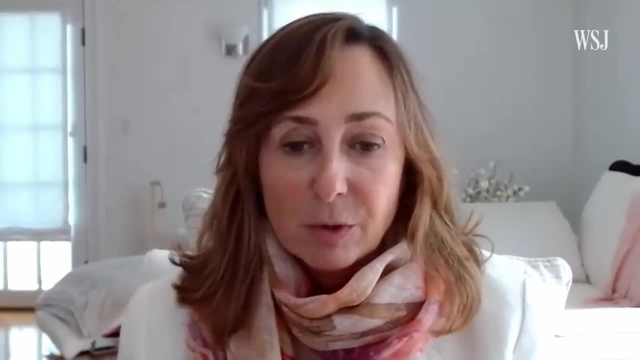 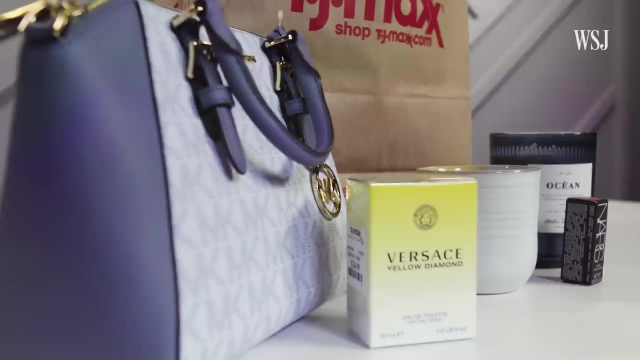 You know, they can cut a deal right on the spot and they can get it to their stores within a week. Department stores, on the other hand, can take weeks to review and approve orders from their buyers. So TJ Maxx buys the merchandise quickly and gets it to their stores within a week. 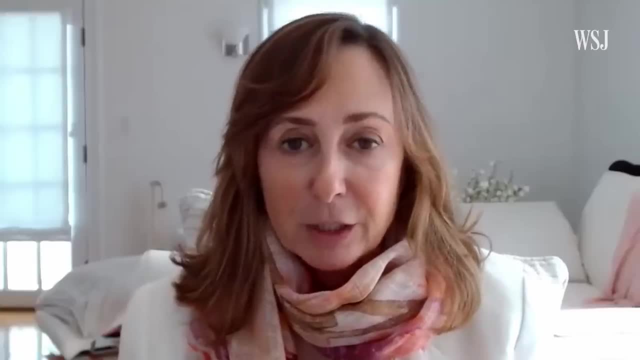 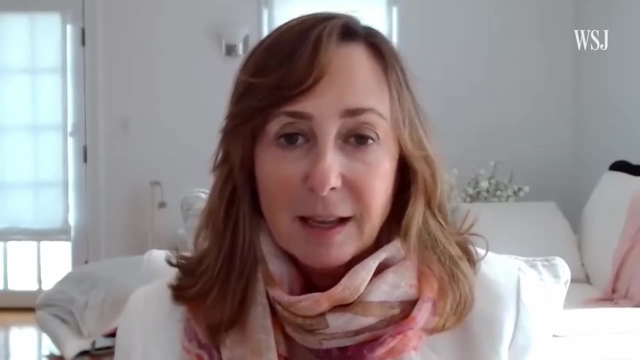 They have a saying internally: door-to-floor in 24, meaning that any merchandise that shows up at a store in the morning has to be on the sales floor by the end of that day. To ensure speed, merchandise often arrives at stores already on racks that employees wheel. 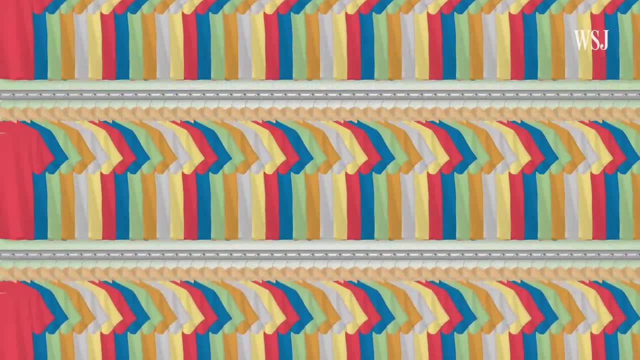 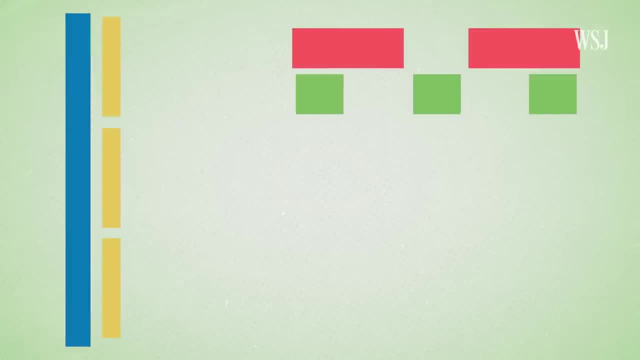 off trucks and move straight onto the sales floor. And once it's there, all the merchandise is laid out differently than other retailers too, helping to create that treasure hunt experience. While most department stores group items by brand, TJ Maxx organizes its